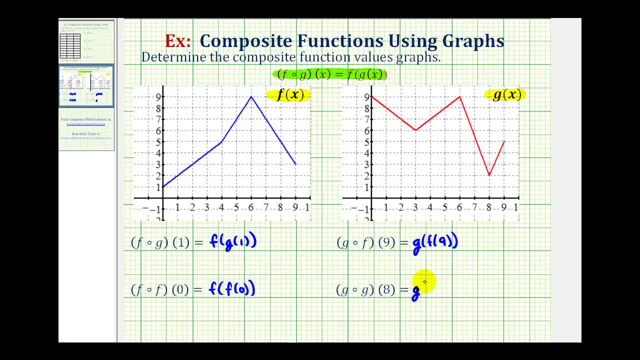 And for g of g of eight, we can write like this: The important thing to remember when evaluating a composite function is to know which function to evaluate first. Using this notation here, I think it's easier to see. we're always going to evaluate the inner function first. 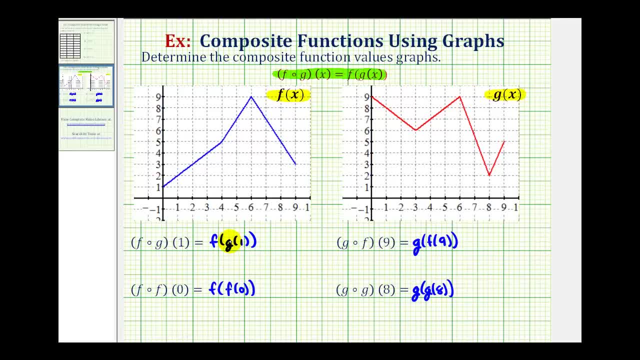 So for this composite function, we'll determine the value of g of one first, And another way to remember this would be to read this as f after g of one. To determine the value of g of one, we need to find the y coordinate on g when x equals one. 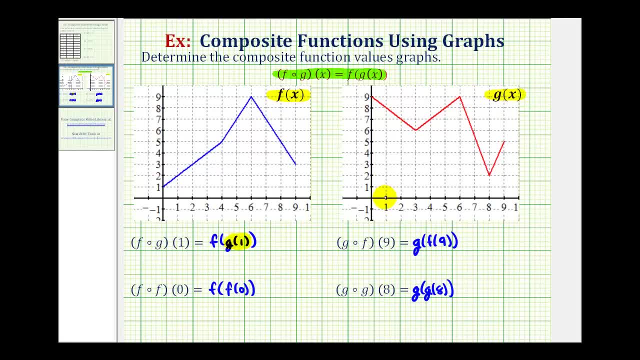 So here's the graph of g. Here's: x equals one. So we go straight to the function. When x is one, notice the corresponding y value or function value is positive eight. Since g of one equals eight, we can write this as f of eight. 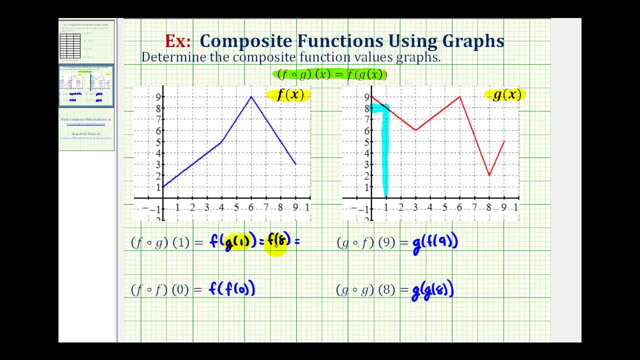 And now we'll go to the graph of function f. Determine the y coordinate when x equals eight. So here's the graph of f. Here's x equals eight. When x is eight, notice the corresponding y value. The corresponding y value is positive five. 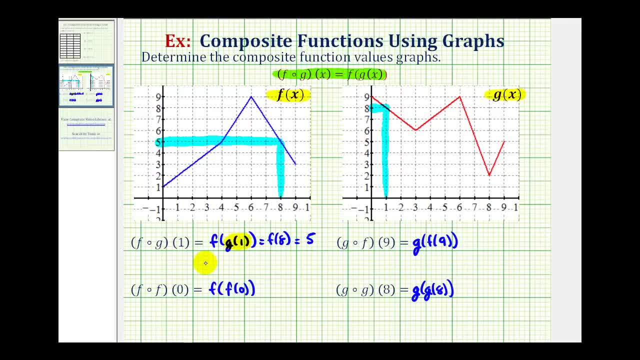 So f of eight equals five. So we can say: f of g of one is equal to five. Next we have g of f of nine. So we'll start by evaluating f of nine. So we'll go to the graph of function f. 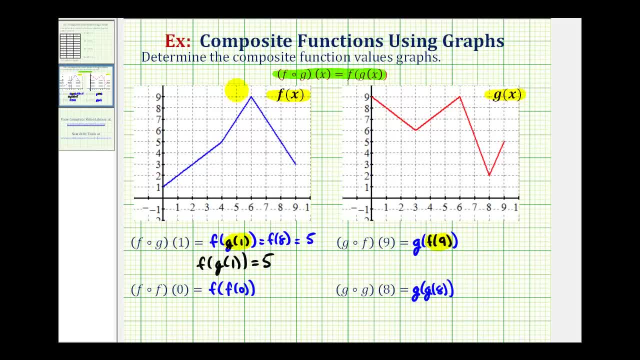 Determine the y coordinate when x is nine. Here's the graph of f. Here's x equals nine. Notice the corresponding y value or function value is positive three, Since f of nine equals positive three. this simplifies to g of three. And now we'll go to the graph of function g. 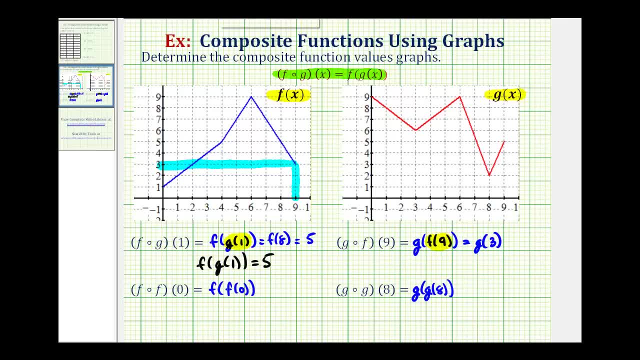 Determine the y value when x is three. Here's: x equals three. Corresponding y value is positive six, which is our function value. So this equals six. So g of f of nine is equal to six. Let's take a look at our last two examples. 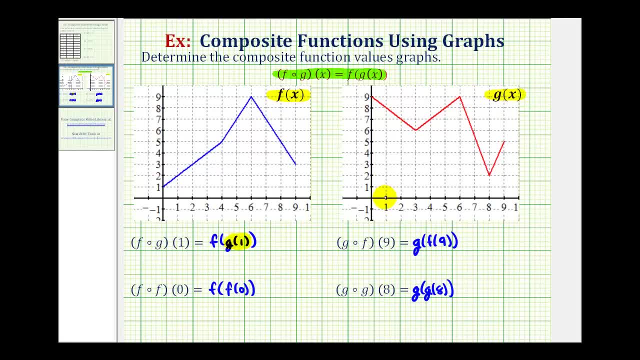 So here's the graph of g. Here's: x equals one. So we go straight to the function. When x is one, notice the corresponding y value or function value is positive eight. Since g of one equals eight, we can write this as f of eight. 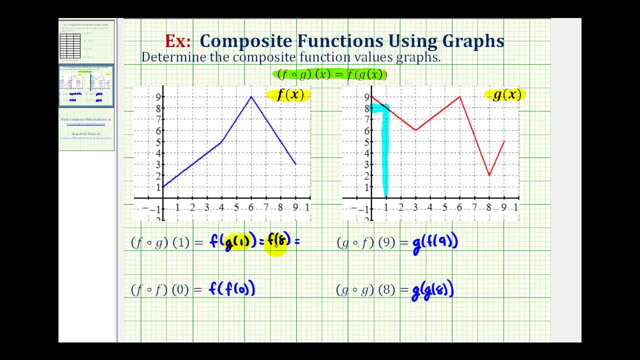 And now we'll go to the graph of function f. Determine the y coordinate when x equals eight. So here's the graph of f. Here's x equals eight. When x is eight, notice the corresponding y value. The corresponding y value is positive five. 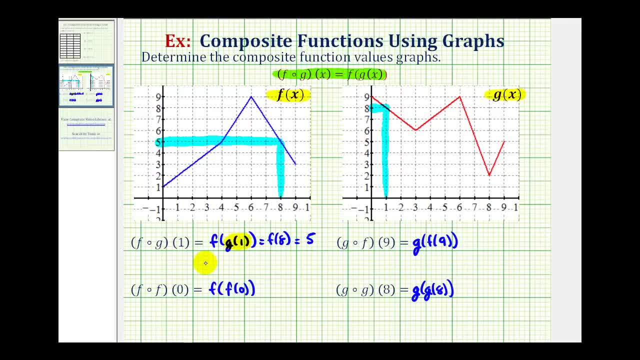 So f of eight equals five. So we can say: f of g of one is equal to five. Next we have g of f of nine. So we'll start by evaluating f of nine. So we'll go to the graph of function f. 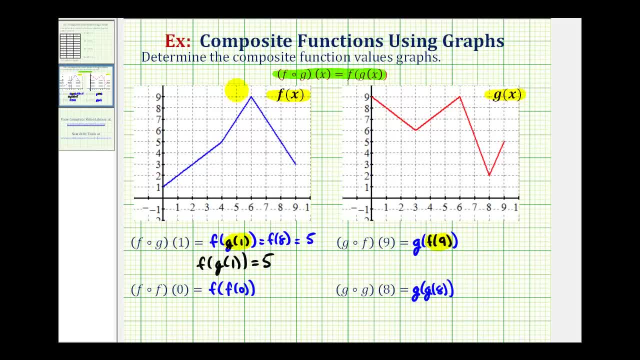 Determine the y coordinate when x is nine. Here's the graph of f. Here's x equals nine. Notice the corresponding y value or function value is positive three, Since f of nine equals positive three. this simplifies to g of three. And now we'll go to the graph of function g. 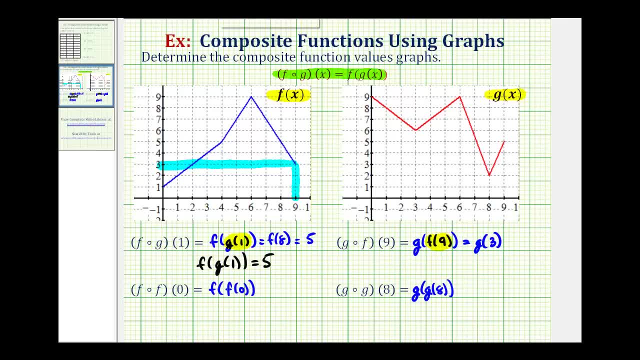 Determine the y value when x is three. Here's: x equals three. Corresponding y value is positive six, which is our function value. So this equals six. So g of f of nine is equal to six. Let's take a look at our last two examples. 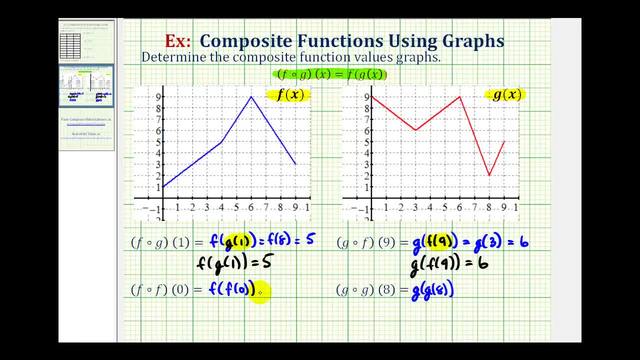 Here we have f of f of zero, And we'll start by determining the value of f of zero. So we'll find the y coordinate when x equals zero for function f. Notice, when x equals zero, we'd be right here on the y intercept. 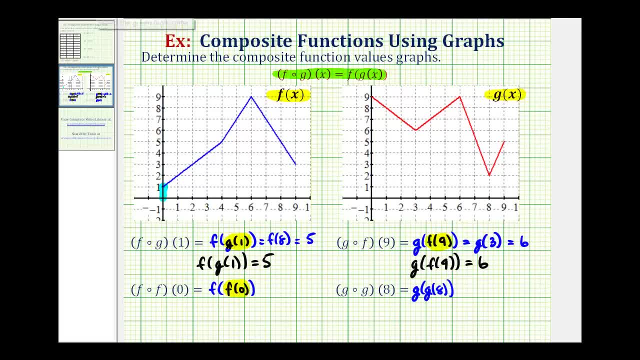 The corresponding y value is positive one. Since f of zero equals positive one, this simplifies to f of one. So using the same graph, we'll find the y coordinate when x equals one. So here's: x equals one. Corresponding y value is positive two.